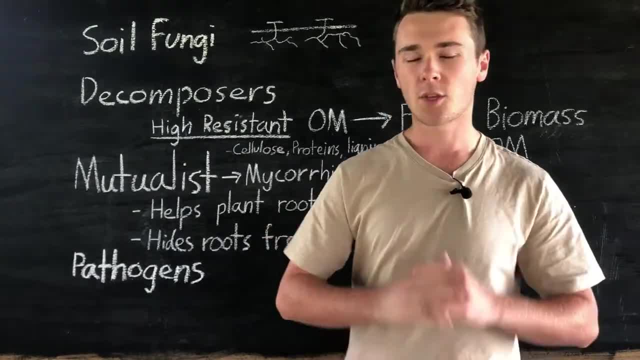 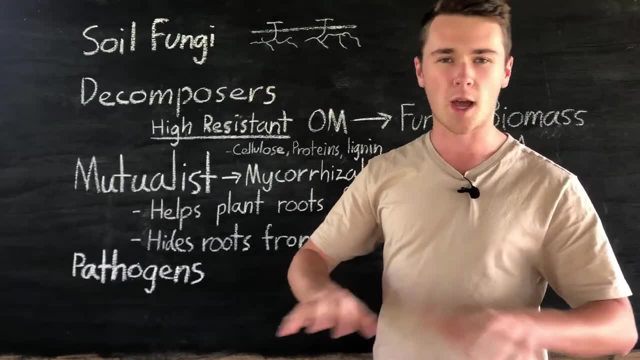 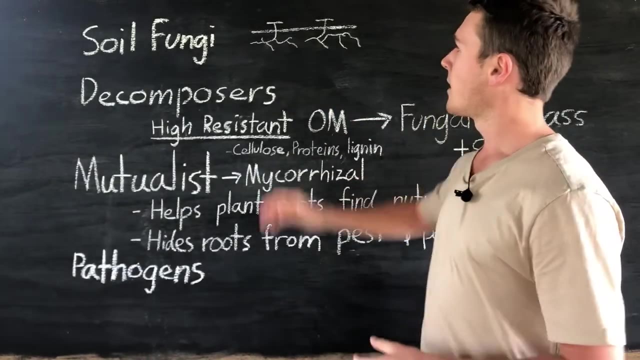 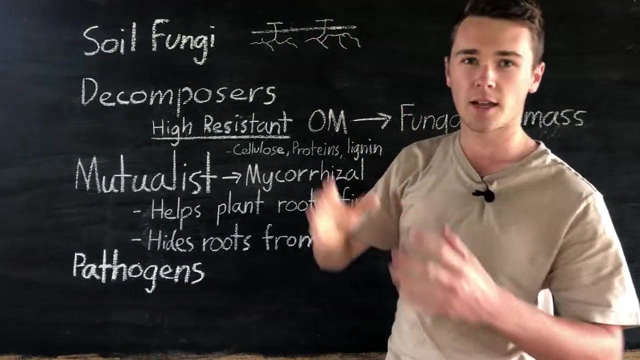 molecules in their environment. So fungi form structures called mycelium, and these are throat-like structures that run mostly under the ground, in our soil or inside organic matter, and then every now and then, when fungi want to reproduce, they pop a little reproductive organ above the ground, such as a. 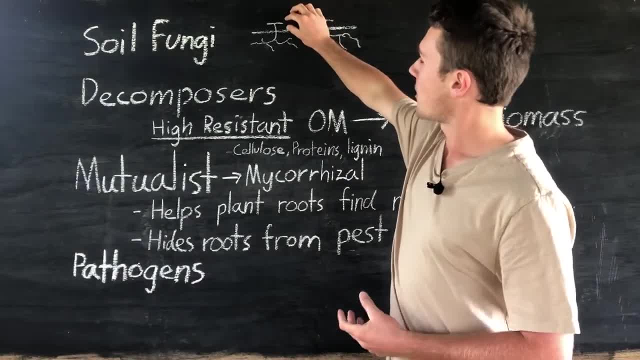 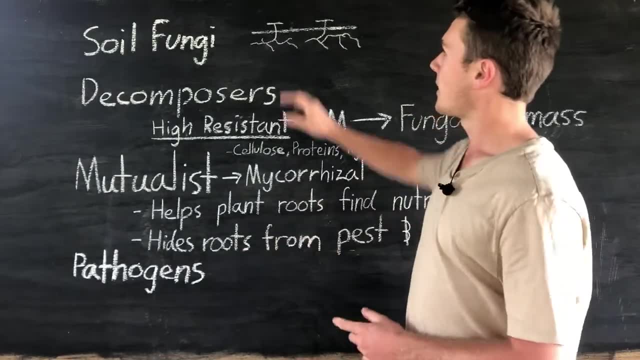 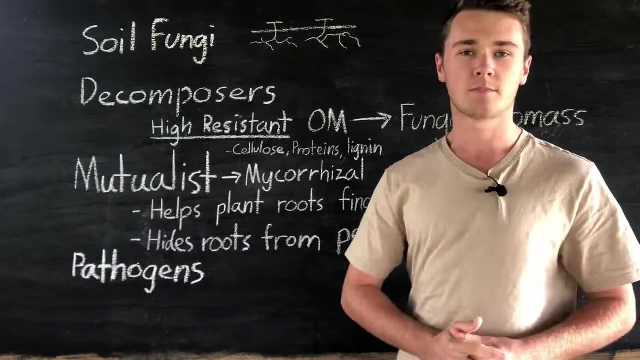 mushroom head, which is represented here, and it releases spores and then these spores pretty much distribute across a land and then they place the spore and then some mycelium grow. So that's a little bit about fungi. Fungi can mostly be separated into three separate groups, or at least in the 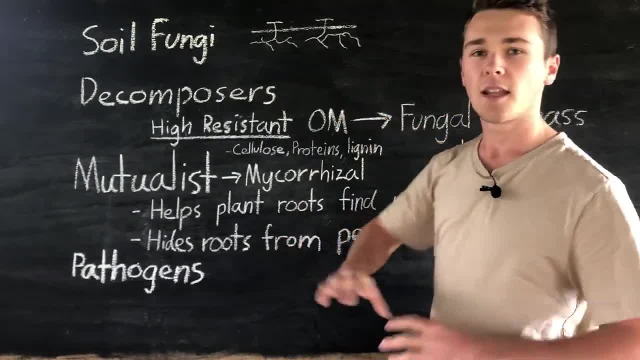 context that we're talking about. So first are the decomposers. Now, this is a really important function for our fungi. So this is a really important function for our fungi. So this is a really important function for our fungi. So this is a really important function for our fungi. 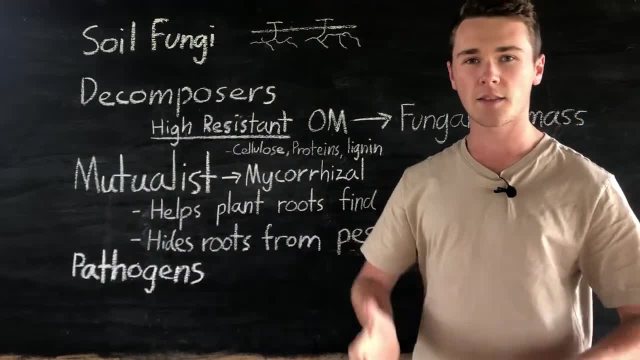 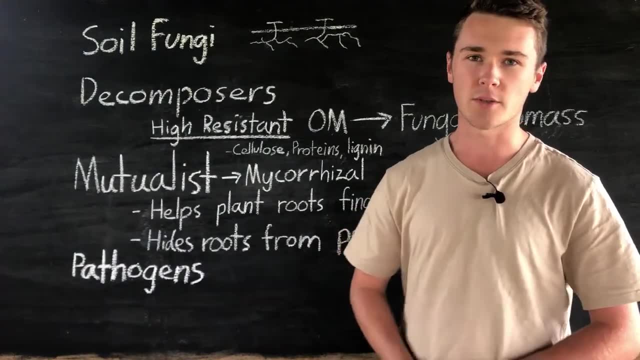 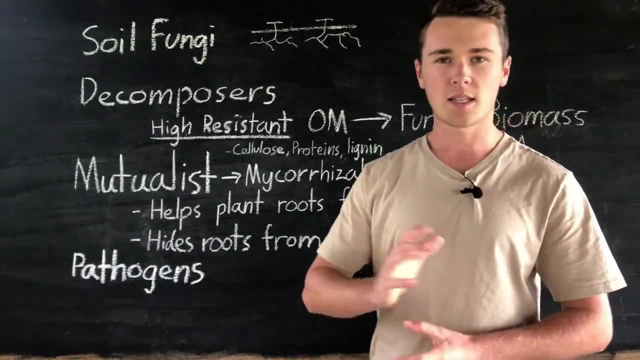 As they break up high resistant organic matter. Now these include cellulose protein and oligolene, all of which have a high resistance to being decomposed. So bacteria, they don't really break down these type of compounds. They stick to more simple structured compounds that are quite easy to break down. 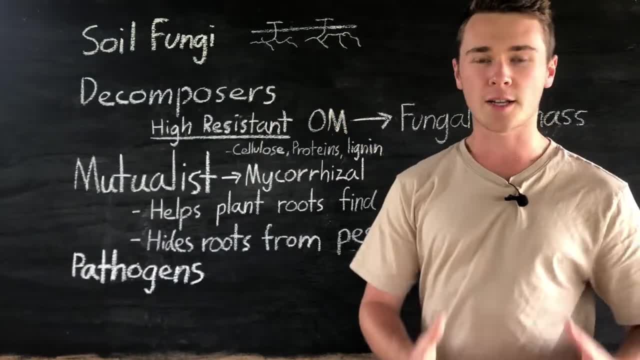 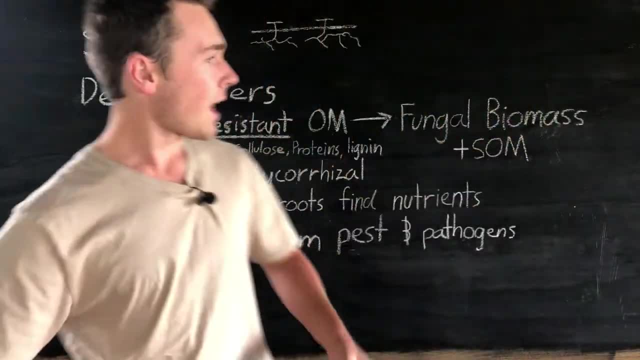 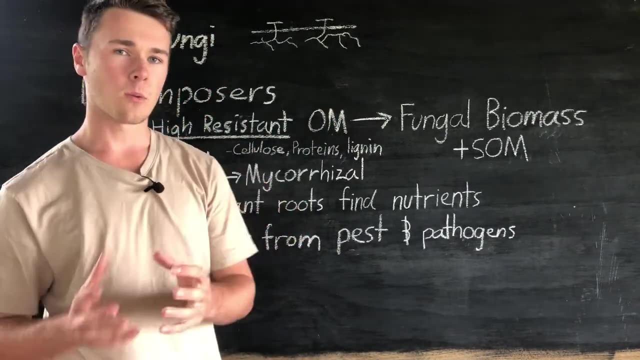 So that's why fungi are really important in the breakdown of organic matter. So the fungi will break down this woody- hard to break down substances- and they'll convert it into fungal biomass. So they'll eat it and then grow their own bodies, Pretty much essentially locking away that nutrients. 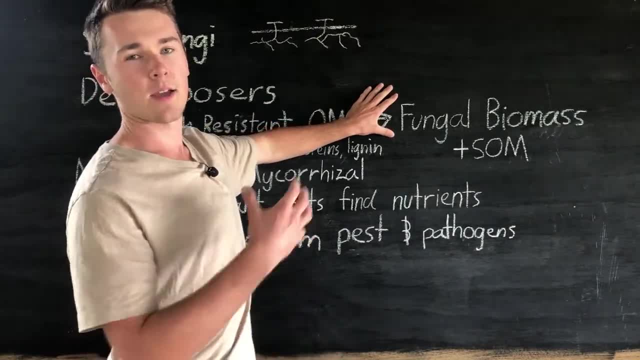 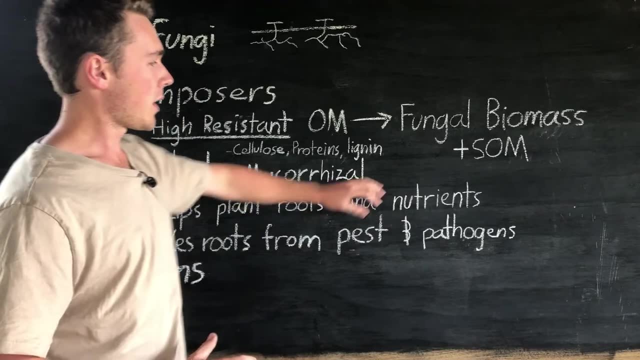 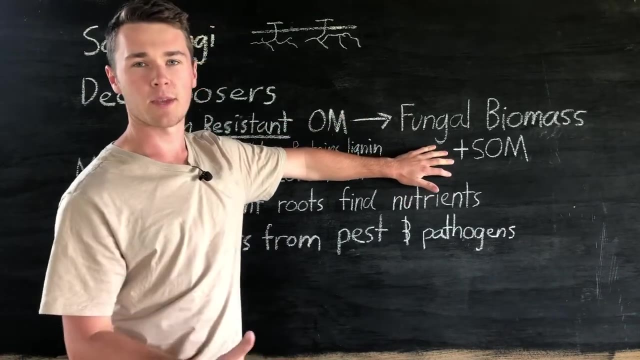 in their body. Now, this is important so that we don't lose our nutrients and then they also form soil, organic matter, which we know from some of the other videos. it's really beneficial for our soil. So essentially, we're storing all this nutrients in our soil as well as building up our soil structure through increasing our soil quality. 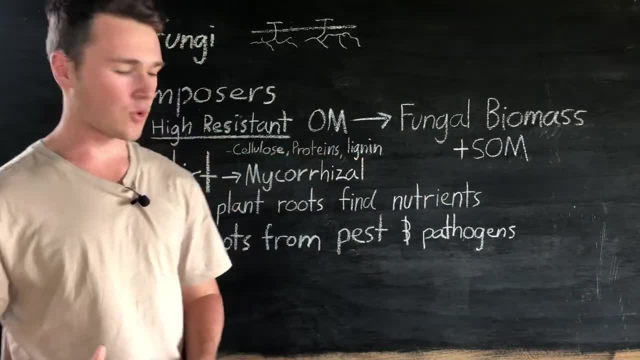 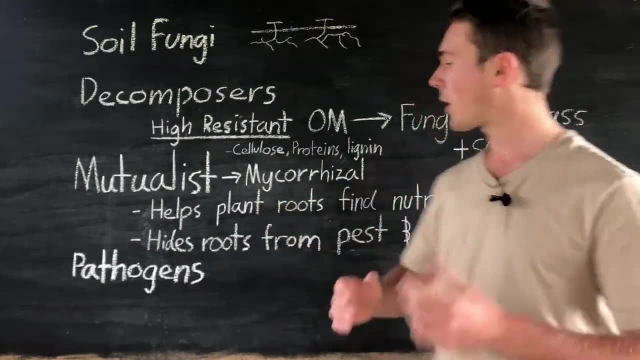 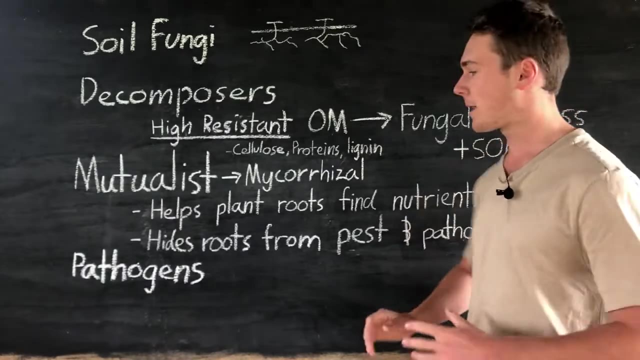 So the next group we can classify fungi in are our mutualist fungi. Now, an example of mutualist fungi are myohysal. Now these: everyone loves these because they support our plants so much. So, firstly, they help our plants find nutrients and 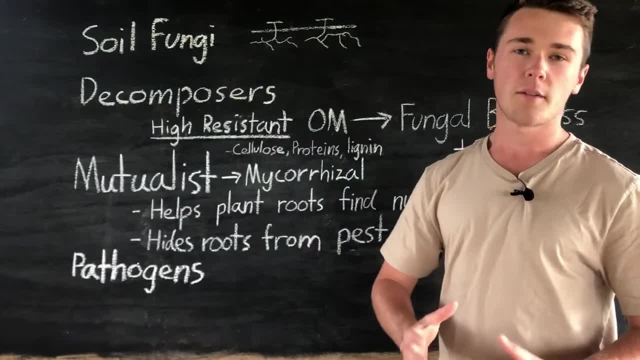 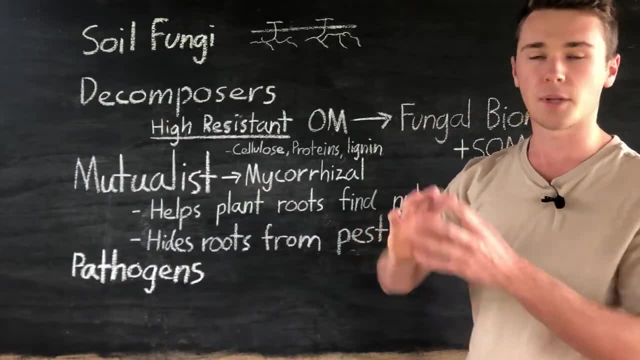 then, secondly, they actually hide plant roots from pathogens and pests, and that's so they pretty much form around our plant roots. So that's the first group we can classify fungi in. and then, secondly, they actually hide plant roots from pathogens and pests, So they pretty much form around our plant roots. 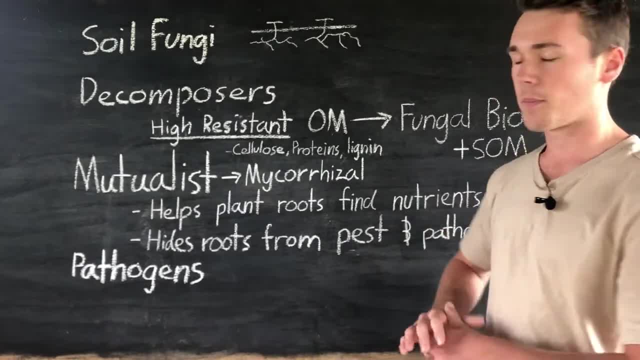 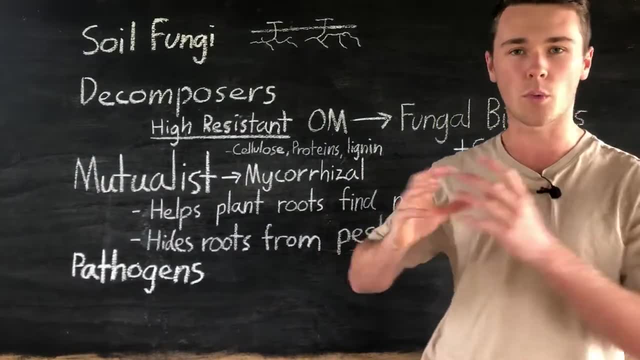 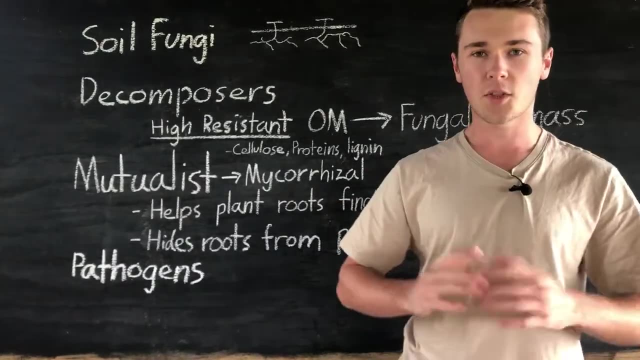 and almost hide them from other pathogens and pests. So an interesting thing about these type of fungi is that they grow with our plants and so the plant benefits and our fungi benefit from this relationship. So this is a really important function for increasing our, I guess, plant uptake of nutrients and 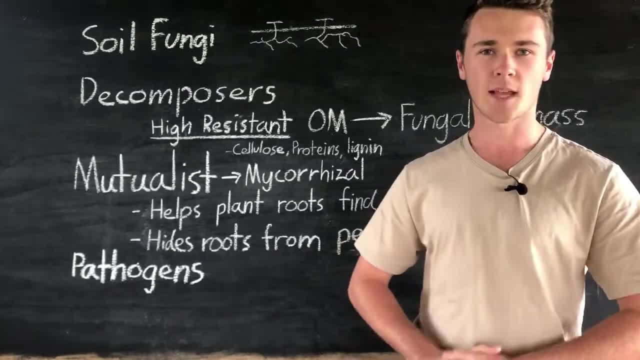 protecting our plants from disease and pests, And so the last group are our pathogens. Now, we don't really want these fungi to be in our soil, So we want to. we don't really want these too much in our soil. we mainly want our fungi for. 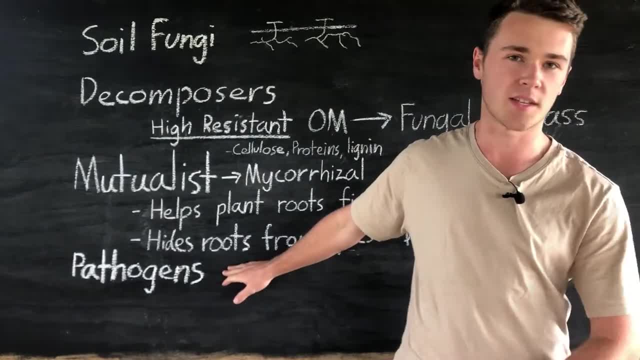 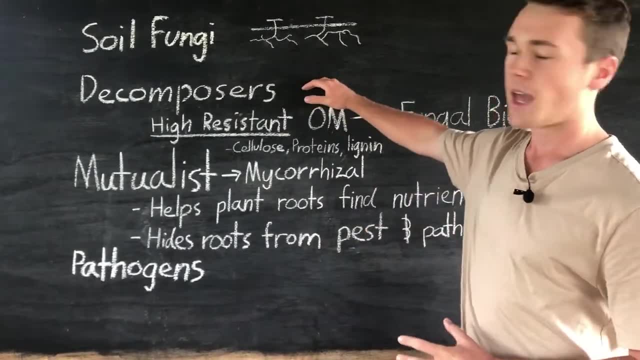 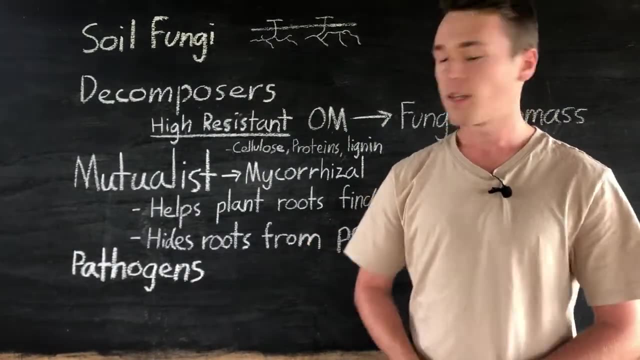 these two groups, But pretty much our pathogens can cause disease in our plants and they can do this by decomposing live plant tissue. So instead of decomposing organic matter, so dead plant tissue, they attack and decompose living plants. Now this can be combated by increasing the biodiversity within. 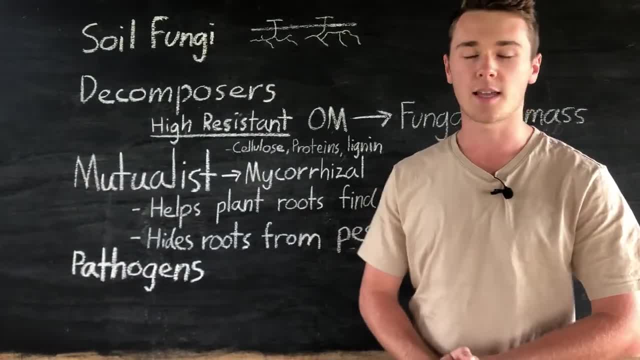 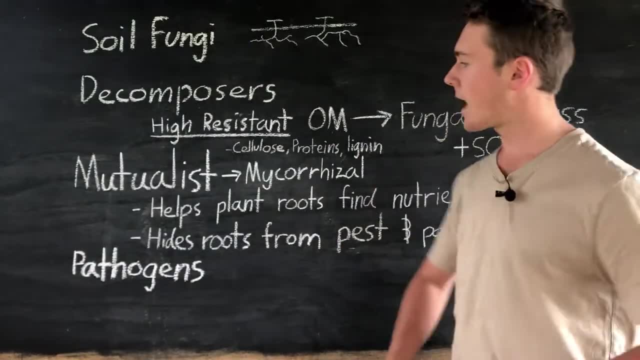 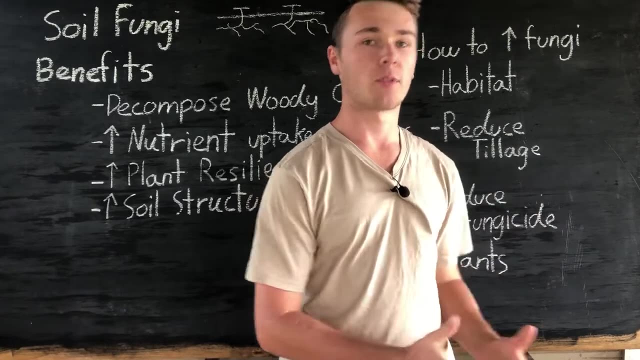 our soil and pretty much what will happen is that our good microbes and our good fungi will pretty much out compete these pathogens, as well as protecting our plant roots and by pretty much growing around them. So now that we know what fungi are and the type of groups that they fall into, let's talk. 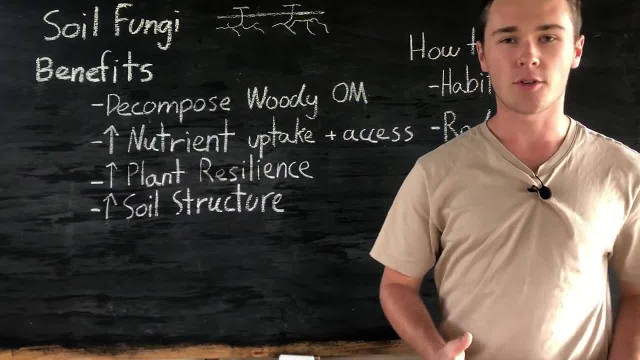 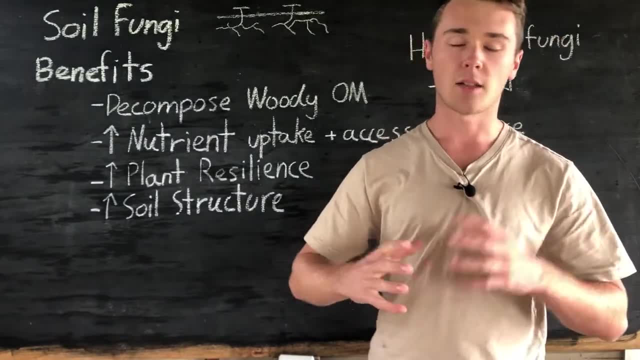 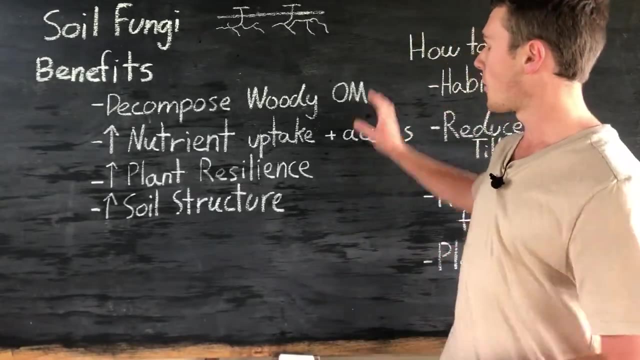 about the benefits. So firstly, they decompose the woody organic matter, like we talked about before. This allows, I guess, the lock up of nutrients, and so they don't get- 해� Hoagland дан贼。. washed away or leached away from our soils. with this we also build up the fungi biomass, which 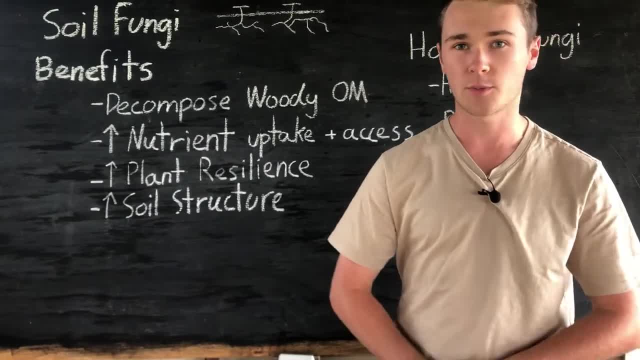 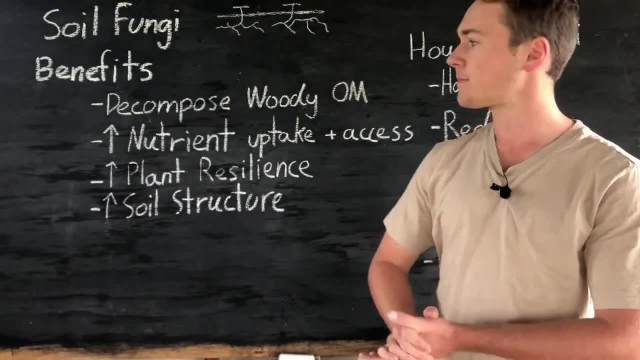 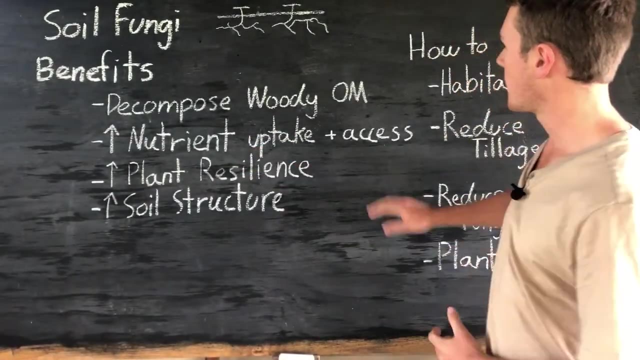 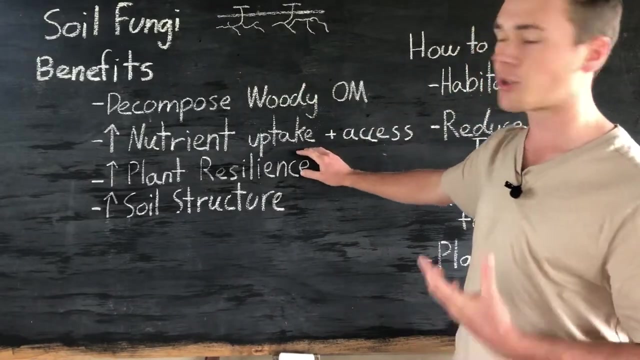 then, when the fungi die or are eaten by nematodes, which we will talk about, i guess, in future videos- it releases these nutrients slowly to our plants. next is that some of these nutrients are released to our plants. so we increase the access to nutrients, but also, with the mutual relationship with our fungi and plants, we can also increase. 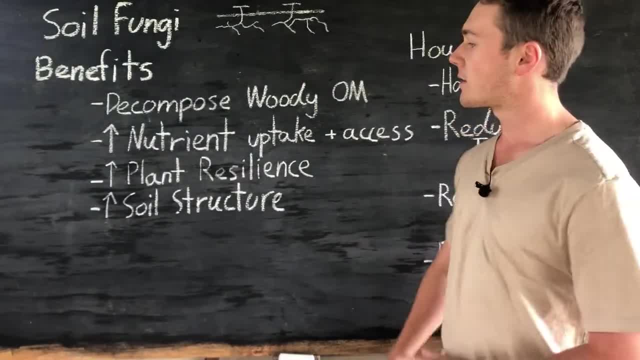 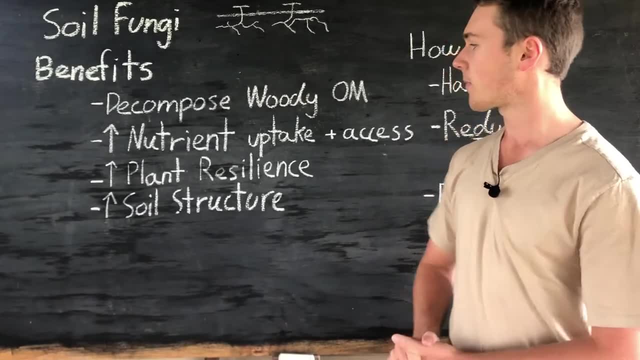 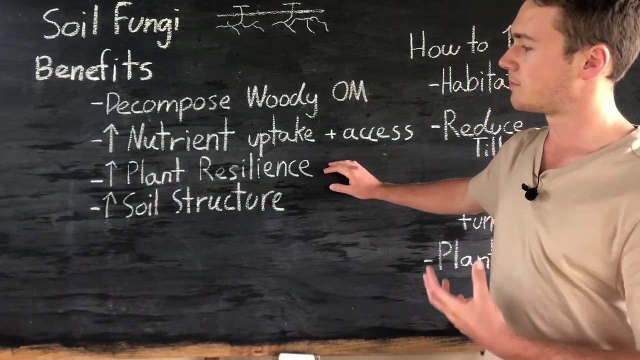 the uptake of of nutrients and so, pretty much, our plants are going to receive more and there's going to be a bigger pool of nutrients in our soil. next is plant resistance to pests and disease. this is massive. we because of this, we don't have to apply as much insecticides or 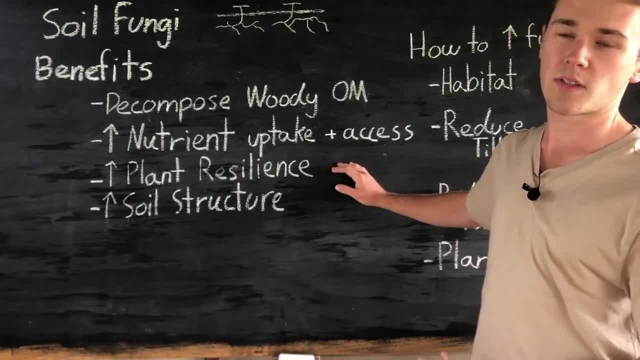 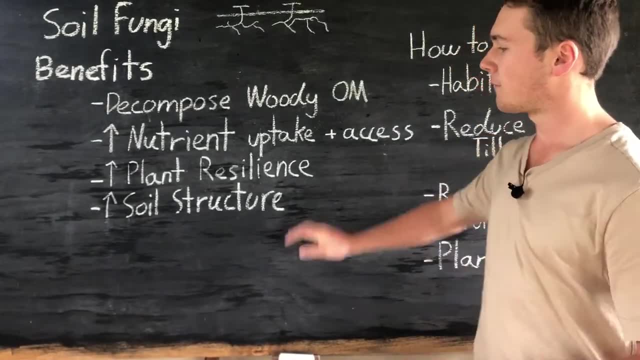 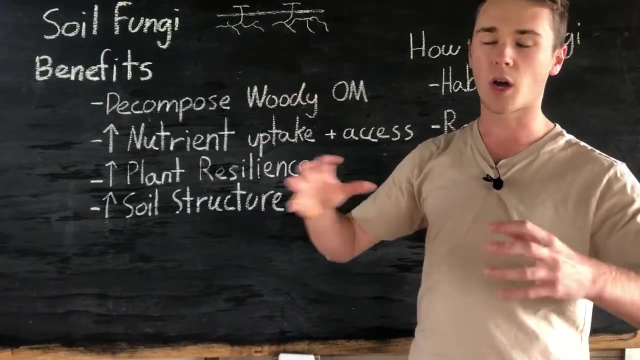 fungicides to protect our plants. we can. we can just use a natural, i guess, competition between our microbes to control population numbers. and then finally, we're going to build soil structure and because we're going to so our fungi, they're going to pretty much hold our aggregates together. 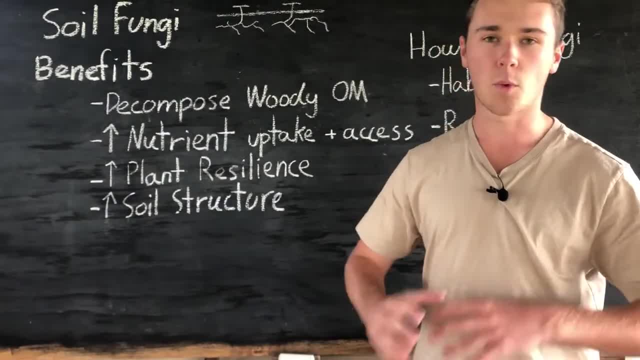 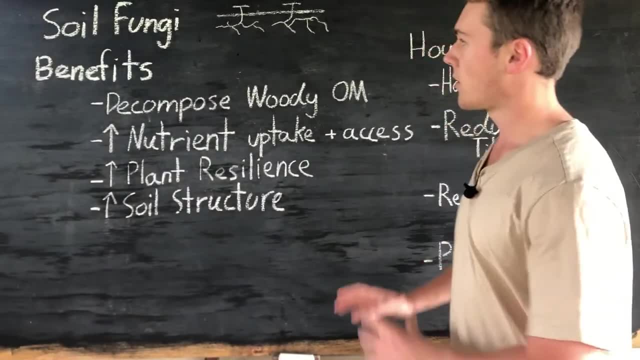 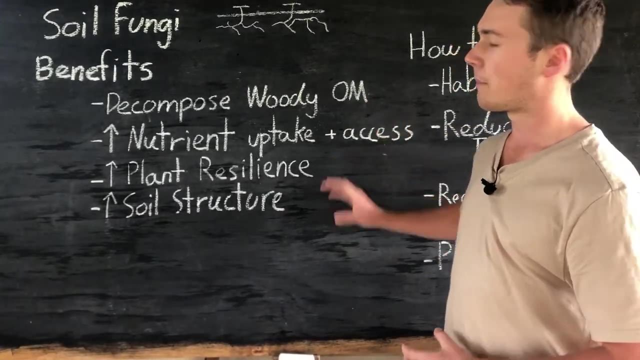 increasing our structure, which will then have a flowing effect that will increase the water holding, the potential of our soil and also increase or improve the drainage. so, overall fungi, there's- um, there's not many, i guess, negatives to it. we're only going to be gaining positives and this is ultimately going to benefit our soil and our enterprise. so now, 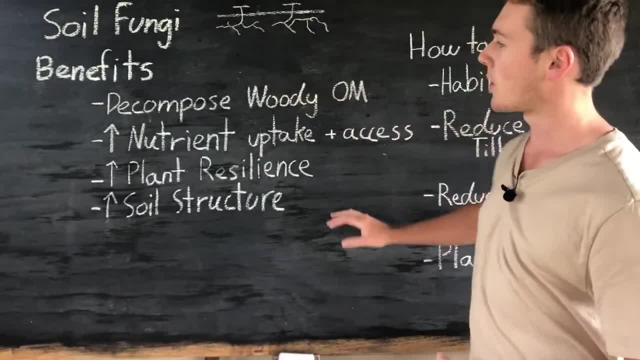 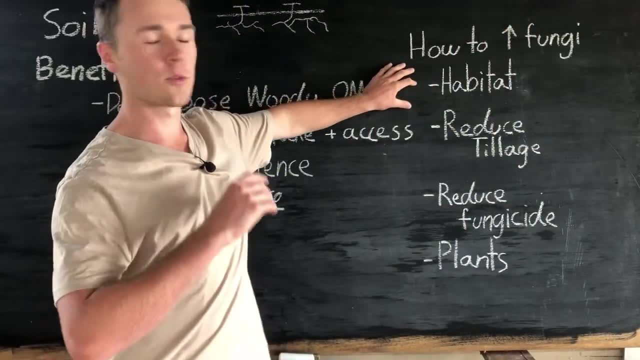 that we know that we really want some fungi in our soil and we want to maximize that, to reap all of these benefits. how can we actually increase our fungi numbers? so, firstly, we're going to um pretty much want them to live in our soil, and so we can do this by increasing 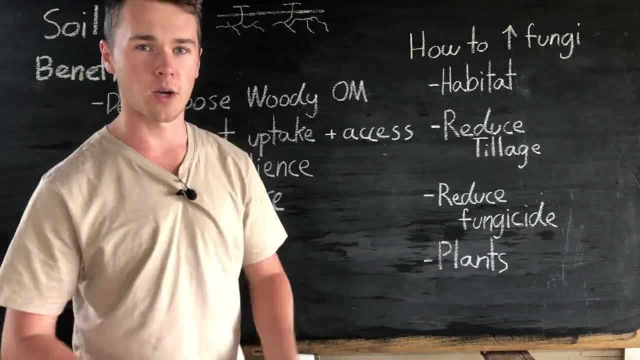 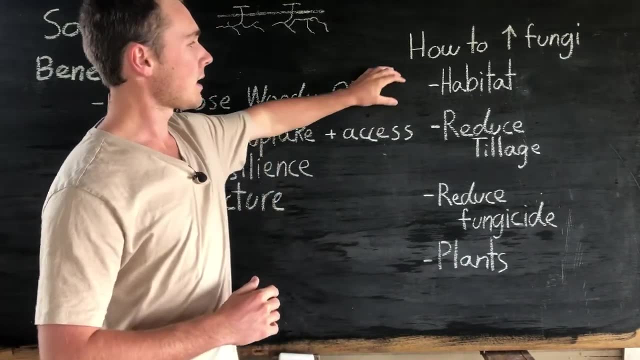 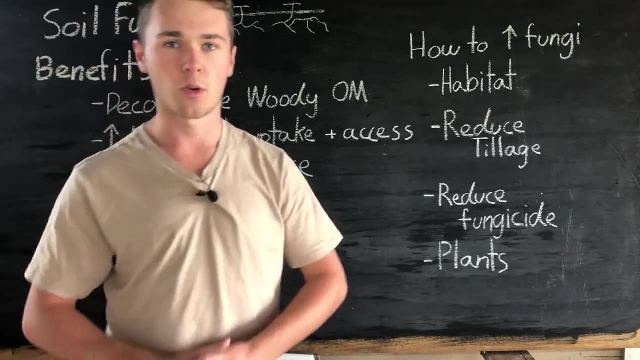 or making the habitat more profitable for our fungi. so fungi love to live in organic matter. that's what they feed off. they love living in, i guess, a nice, safe environment surrounded by, surrounded by plant roots. so that's exactly what we want in our soil: lots of plant roots, lots of. 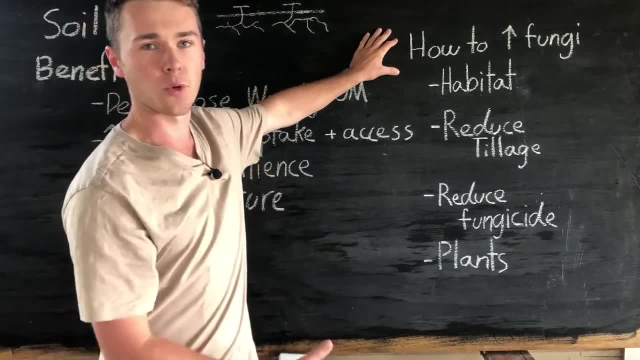 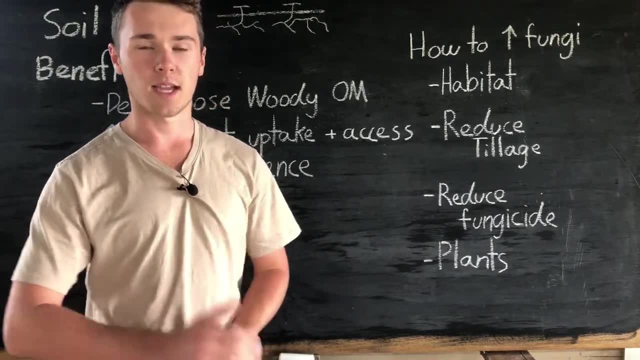 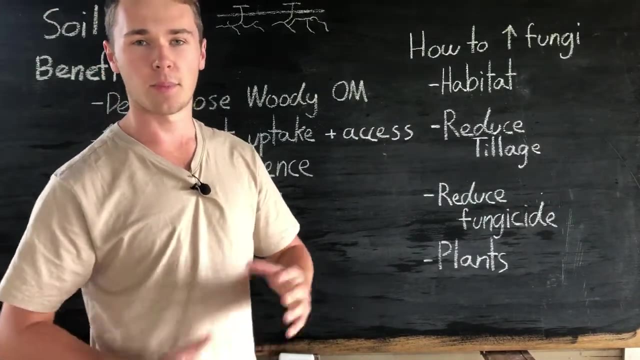 organic matter for these fungi to have lots of food and to grow. now, they don't like lots of sunlight. sun can damage them, so we want to make sure we have lots of ground cover- um, and we have. we also have another video about plant carbon, the benefits of that, so check that out. but in this um sense, we 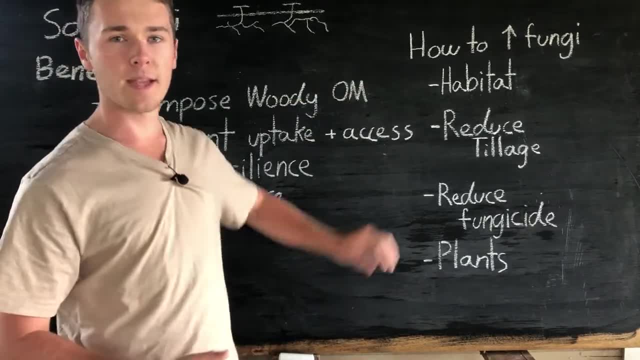 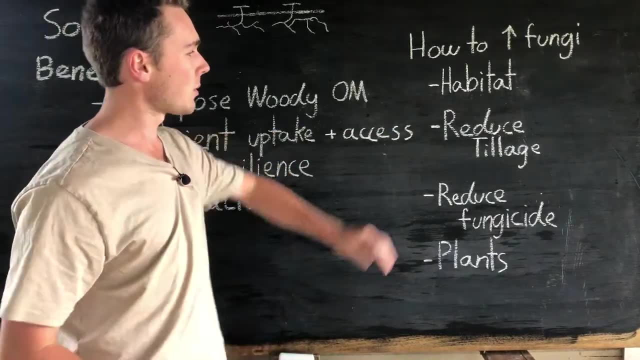 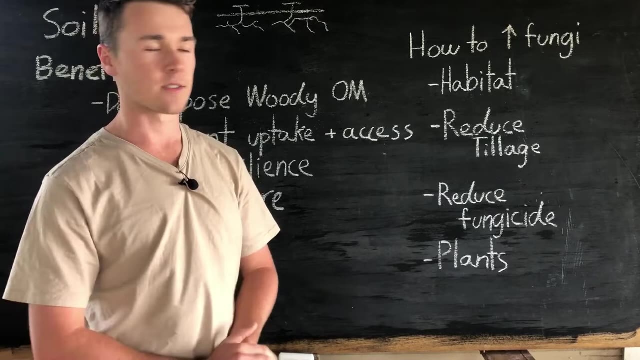 want lots of ground cover to protect our fungi. next, we want to make sure that our fungi aren't being, i guess, ripped apart or the mycelium that spreads through our soil isn't getting cut up. so we're going to reduce our tillage, and we can do that with no till or reduced till type of strategies. 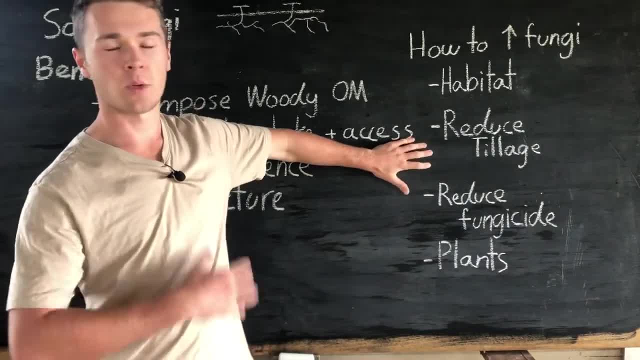 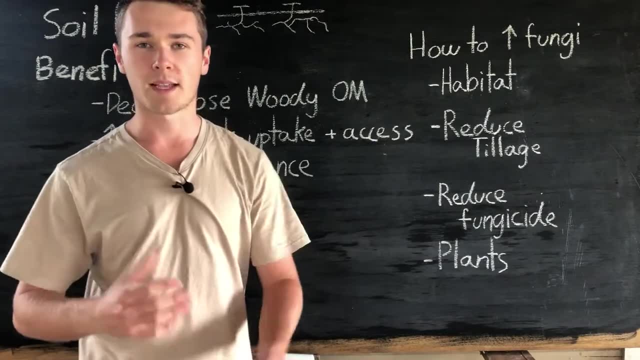 and so this will promote growth and will prevent, i guess, setbacks of our hunger. next, we're going to reduce um fungicide. now this kind of makes sense. if we're, if we want to promote fungi, we don't really want to be applying uh fungicide which will kill them or hurt them. 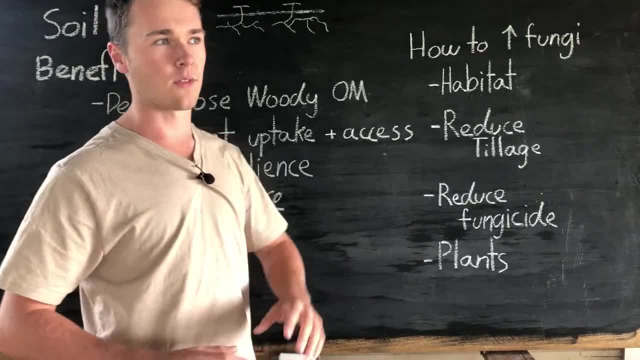 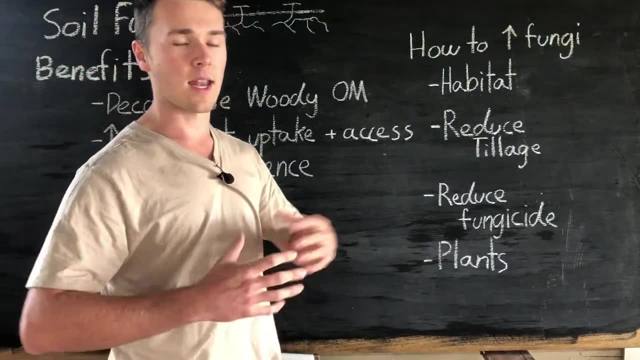 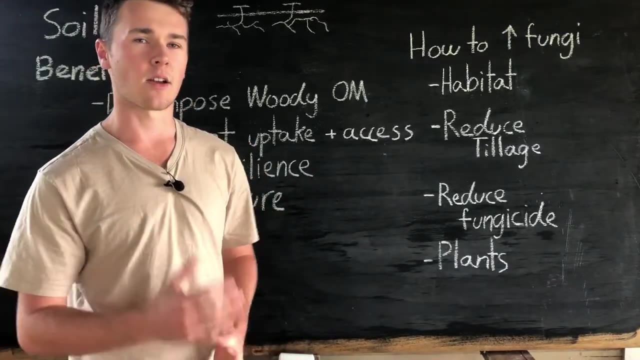 now this is more in the sense of broad spectrum fungicides which if you apply across a whole paddock it will damage all your fungicides. if you do have a um, say an outbreak of rust or some disease like that, applying a um, a fungicide like that is almost a necessary evil. 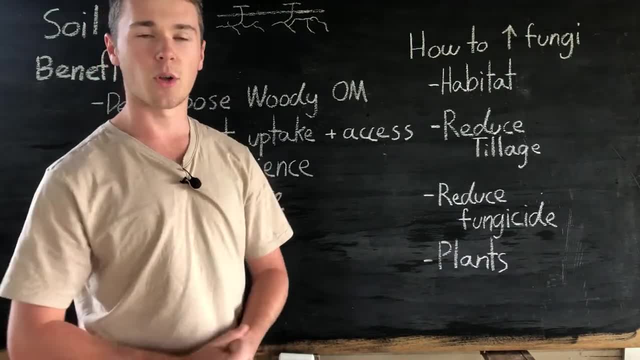 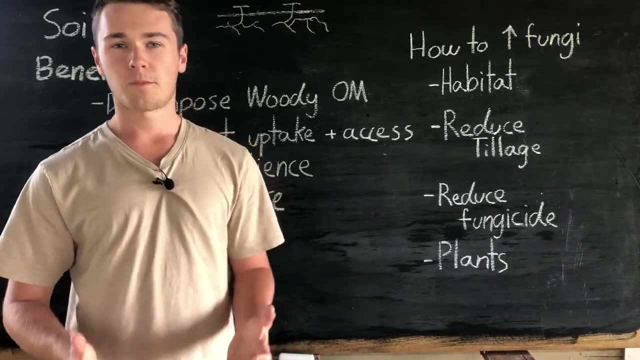 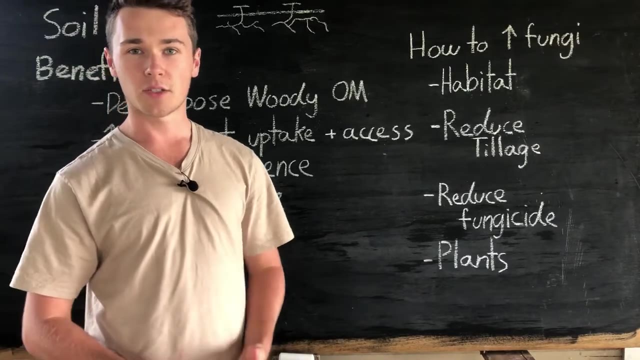 um, that you have to do unless you set up a really good ipm or integrated pest management at the controllers, which we should always be looking to do. but if a population of pathogens get out of control, you know insecticides or herbicides will. fungicides are a great way to. 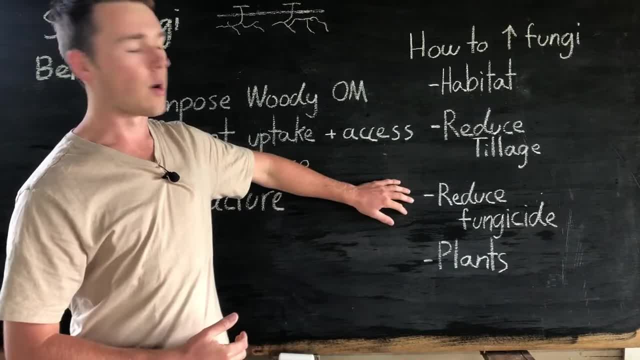 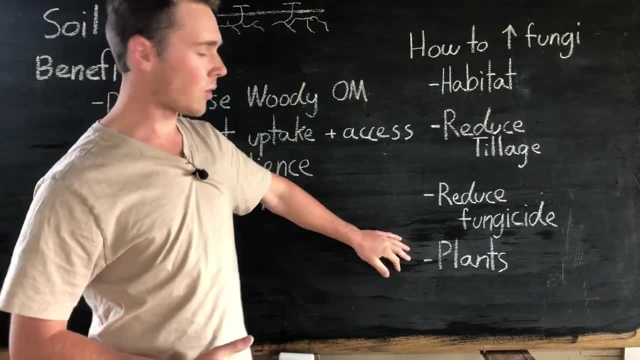 control that. we just have to understand the negative impacts that they'll bring in fungicides and that's why we want to make sure that we have fungicides in our soil, because if we have fungicides in our soil it will damage our fungi in our soil. and, lastly, we want to make sure the plants that 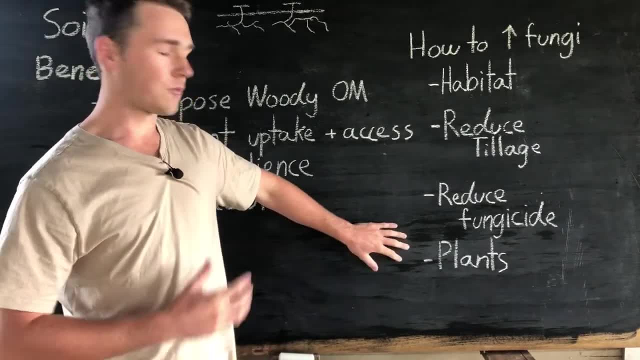 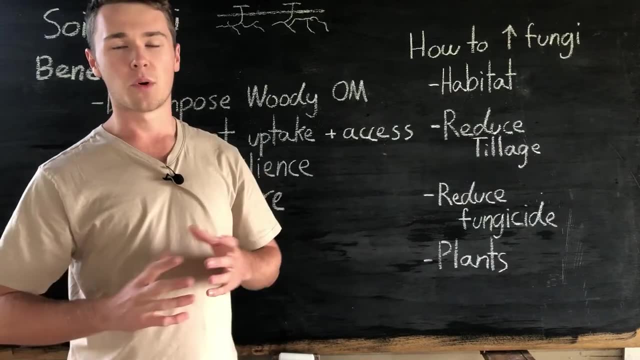 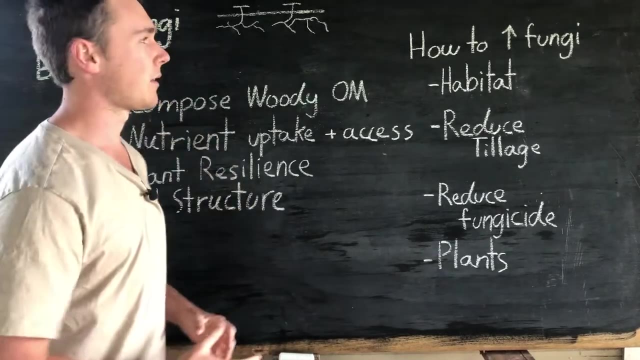 we have in our field really support the fungi growth, so some of these can be legumes and grasses. the roots on these fungi love to live in between them and amongst them, and so having plants that they really like will pretty much want them to live in our soils. now, fungi and all our band of 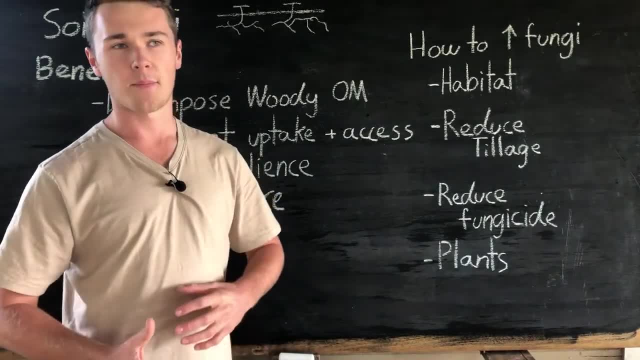 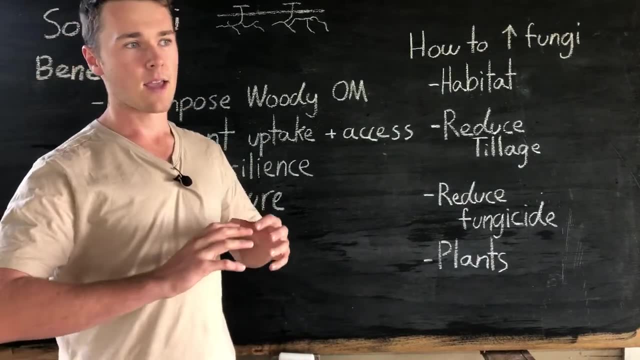 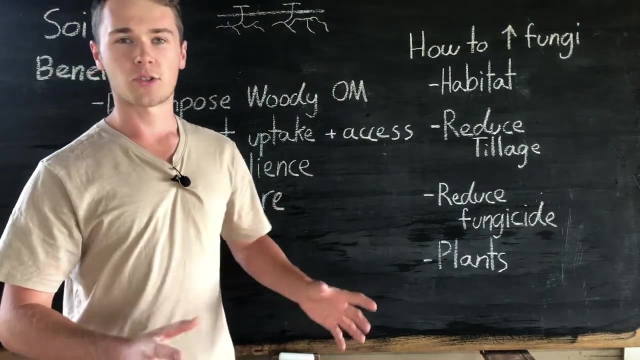 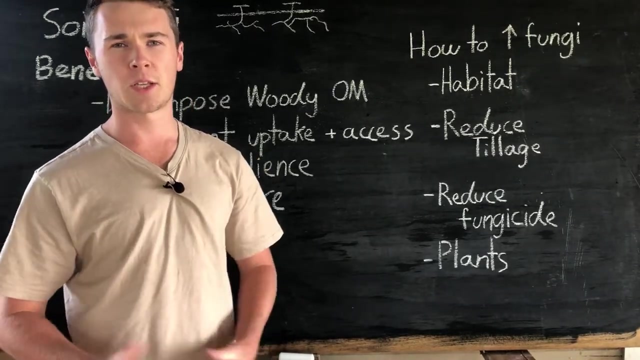 plants are very hard to live in and so if we have a pretty good um and we can spread that across our paddocks or our fields to increase or introduce different populations. but essentially what we can do is buy inoculated soil or um or grain and put it across. your farm, otherwise you can make compost. you can make your own compost or compost tea which will have your fungi and some other microbes in there- anything really to introduce and get the numbers there. but other than that you've got to make sure that they have the environment that they want to. 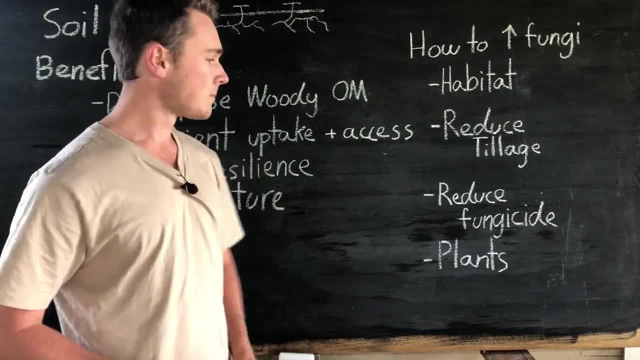 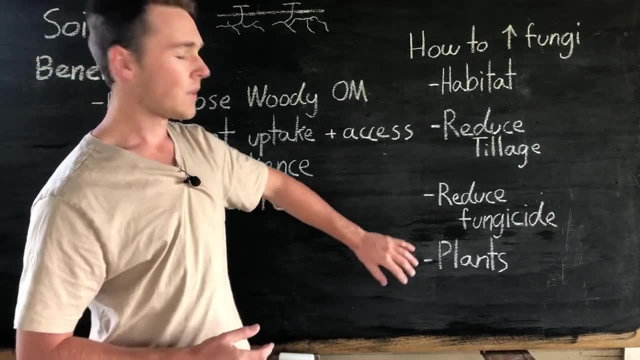 live in. otherwise they're going to die off or or not want to be there. so just because you're you're pouring really rich, micro rich compost tea across your field doesn't mean that they're going to stay there or survive. we want to make sure we're doing all these things to really make the